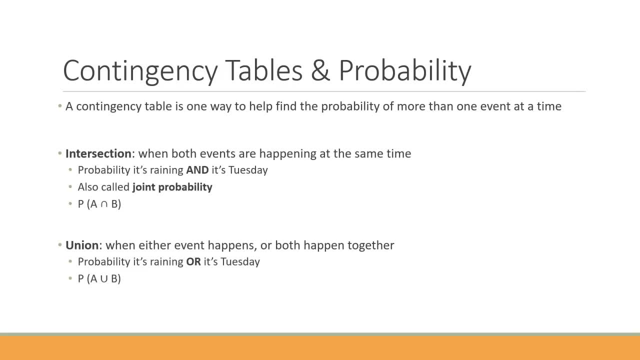 intersection is when both events are happening at the same time. So, for example, that's the probability that it's raining and that it's Tuesday. So this can also be called joint probability And we'll write it out like this, with the probability of A and B. So that little. 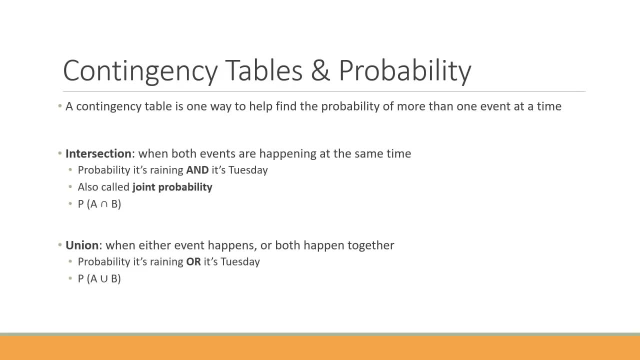 upside down. U is our and sign A. union is when either event is happening or they're happening together. So, for example, it's the probability that it's raining or that it's Tuesday. Right, It doesn't have to rain on Tuesday. Both events don't have to happen together. 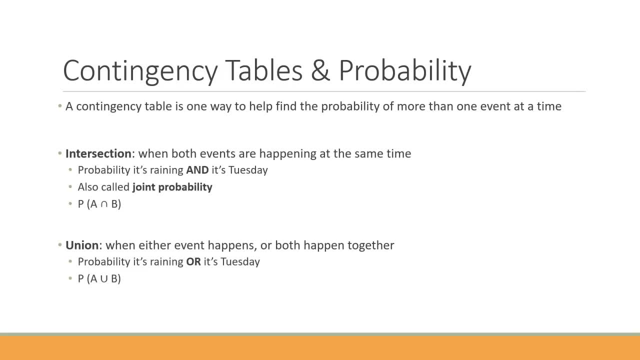 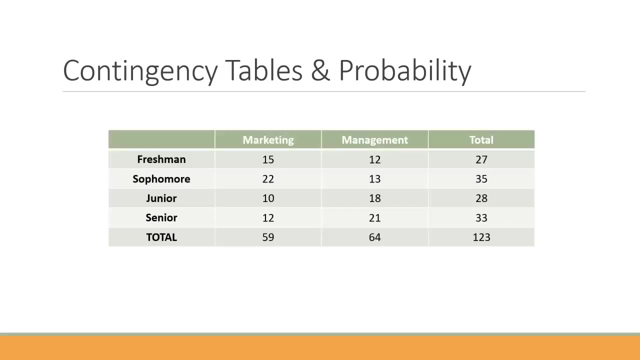 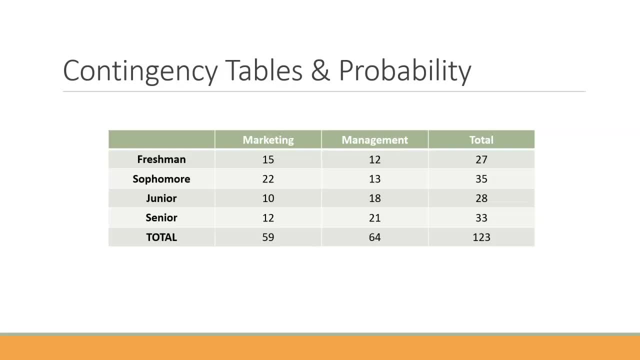 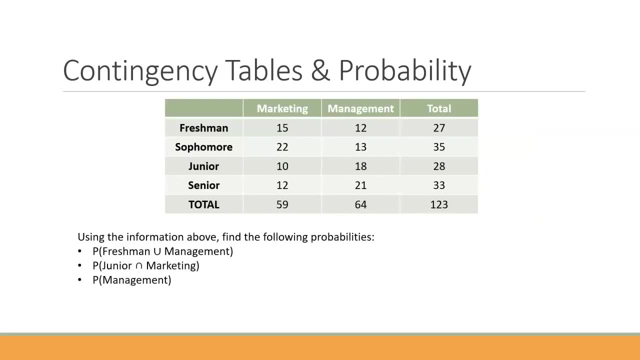 We have freshman, sophomore, juniors and seniors, And then we have a couple different majors. We have marketing majors and management majors. With this contingency table, we can find the following probabilities: First, the probability of a freshman or a management major, Then the 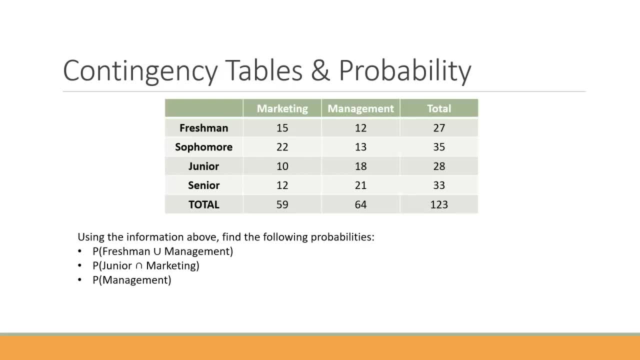 probability of a junior and marketing major And then just the probability of a management major. So let's first talk about the or Freshman or management. It's always helpful to then highlight the pieces that we care about, And that's these here: The freshman row and the. 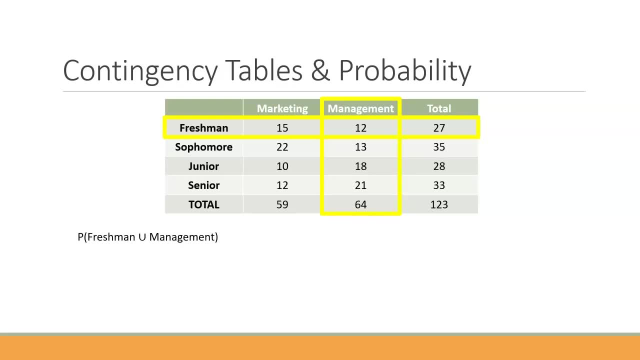 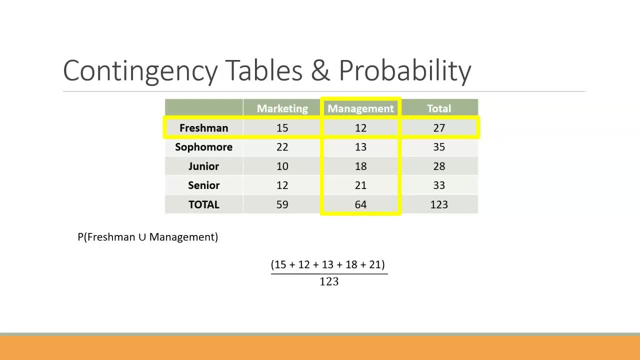 twice, Right? So there's a reason why we can't just go 64 plus 27 and take the two totals here, Because that would count the 12 twice. So instead think of it as just adding together all of the individual pieces, The 15 and the 12.. And then we work our way down the management column.